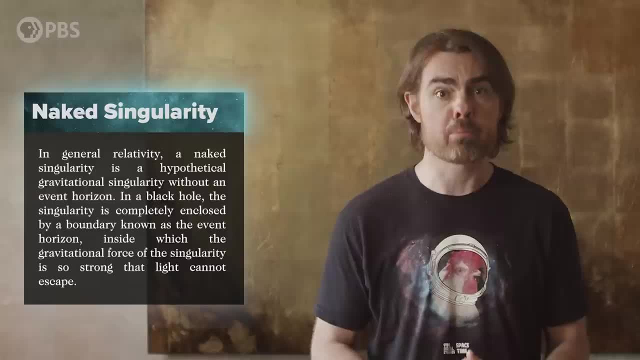 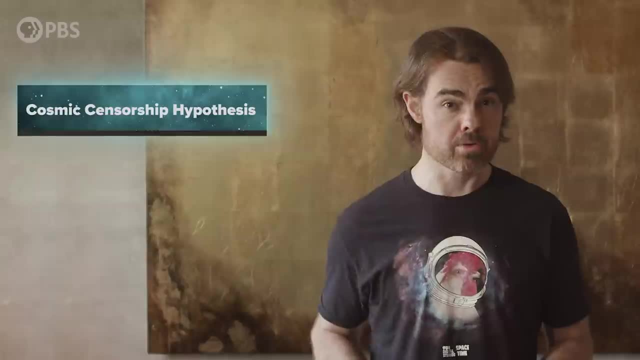 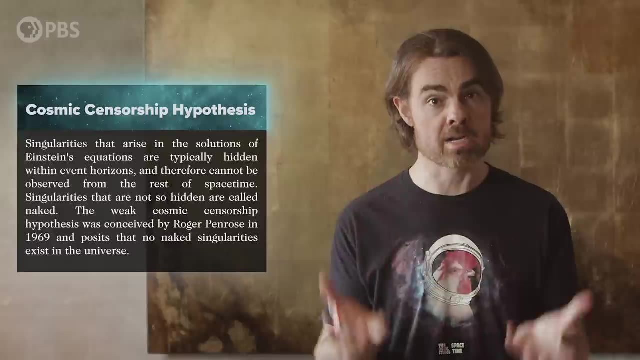 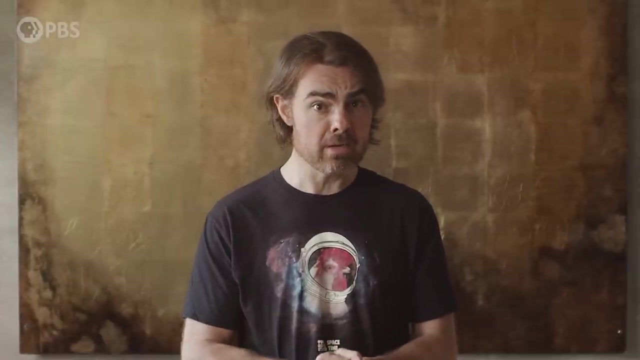 wreak havoc on our understanding of causality and our precious laws of physics would become unhinged. Given the dire consequences, Roger Penrose proposed the cosmic censorship hypothesis, which basically states that every gravitational singularity must be surrounded by an event horizon. In an upcoming episode, we're going to look deeper at why many physicists believe the 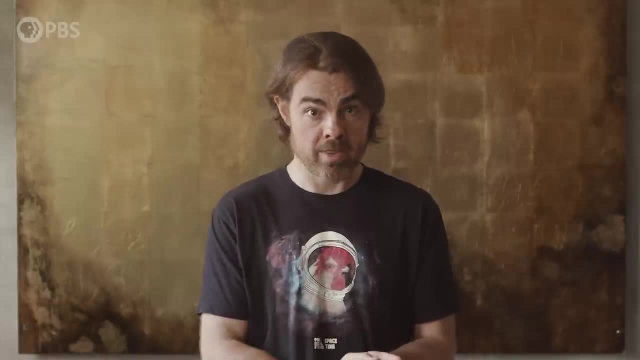 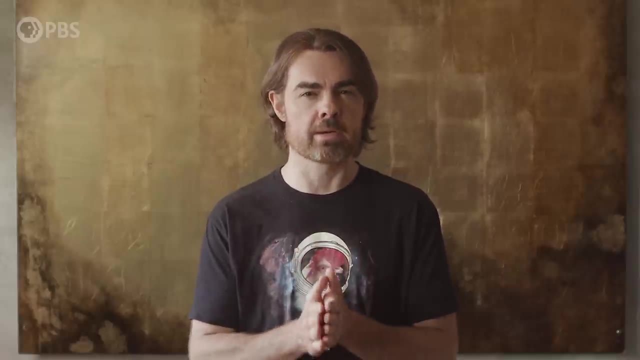 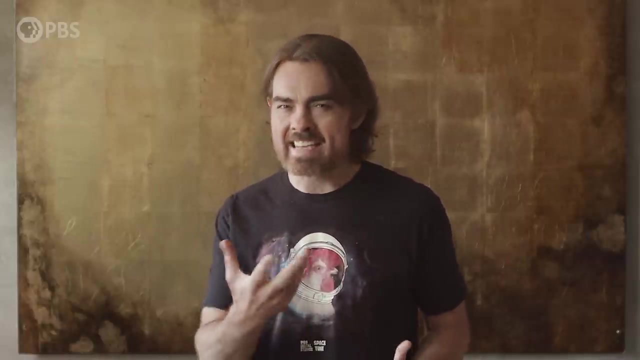 cosmic censorship hypothesis must be true, even without knowing exactly why it's true, and we'll see why other physicists have begun to doubt its validity. But today we're going to look at astrophysics and see how exactly a naked singularity might. 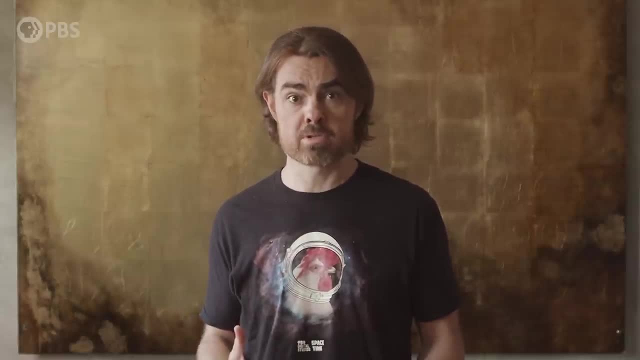 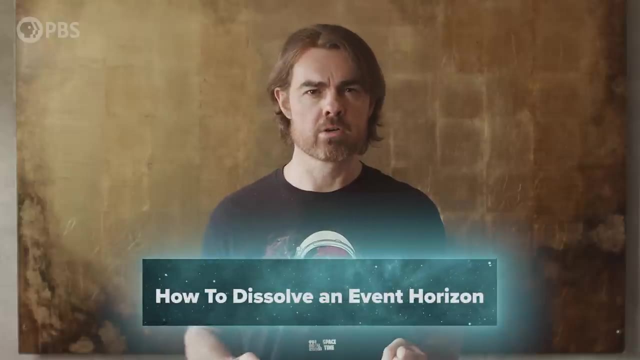 be formed in the first place and how the universe seems to work very hard to protect itself from them. So let's talk about how to dissolve an event horizon, Although I would ask you to please not try this at home, for the sake of all of physics. 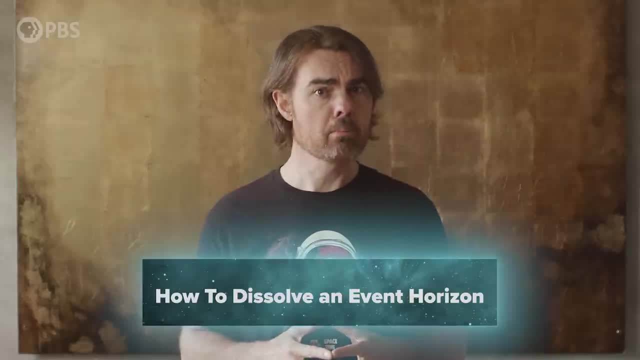 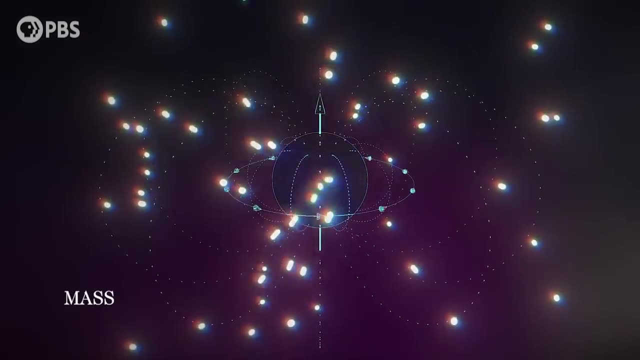 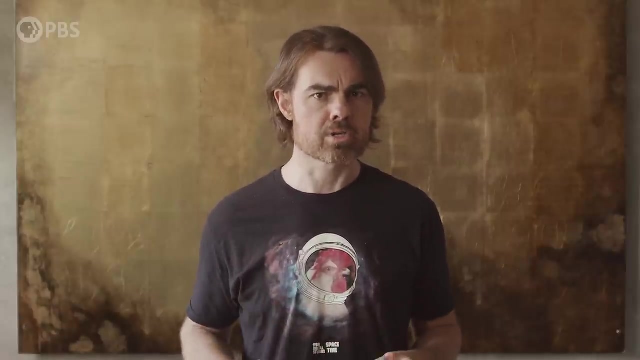 According to the so-called no-hair theorem, black holes can have only three properties – mass, electric charge and spin. Mass is what makes a black hole a black hole, and so the simplest black holes have only this property. These are Schwarzschild black holes, and with only mass that means they also have inward 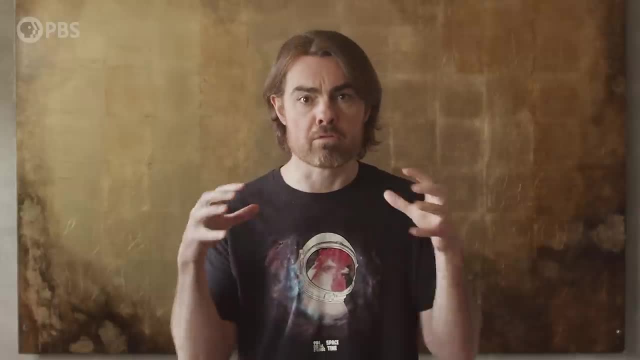 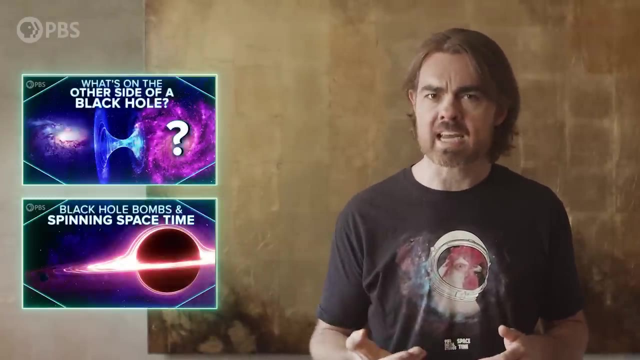 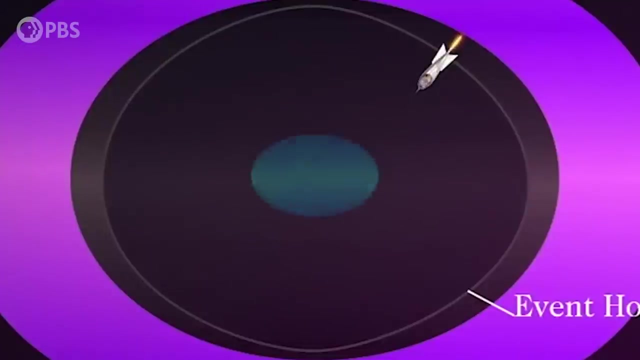 pulling gravity With nothing to counter the inward pulling. they are called black holes. In recent episodes we also explored the rotating, or Kerr, black hole. Inside we found that the rapid rotation has spun the point-like singularity into a ring of infinite density. 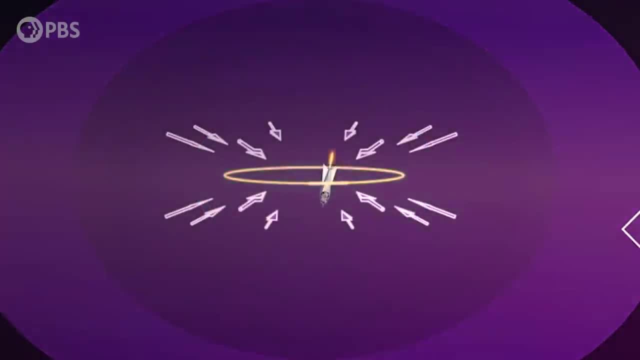 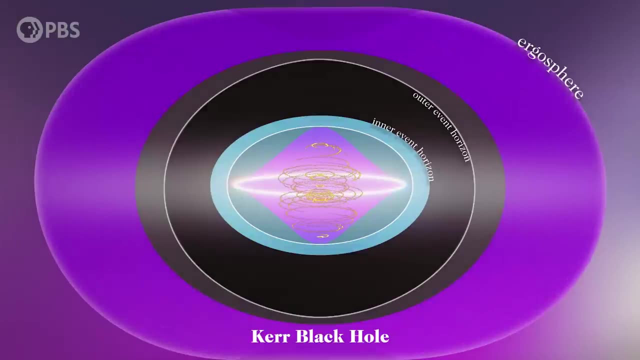 The time machine is on the other side of that ring. by the way, The same rotation that forms the ring also drags the fabric of space into a vortex, which counters the inward pull due to the singularity spin. So let's get started. 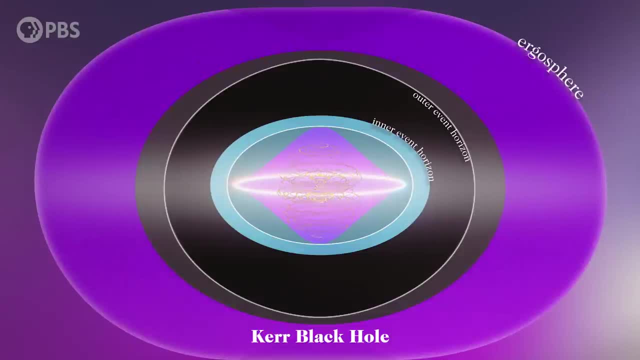 The result is that we get this region around the singularity, where the faster-than-light inward flow of space is halted. It's like the eye of the storm and it's separated from the surrounding cascade by the inner event horizon. As the spin of a Kerr black hole increases, the spacetime waterfall is beaten back and so the inner horizon grows At a certain, very high rotation rate. the inner and outer horizons merge, which means they both vanish. There's no longer a region where the inward flow of space exceeds light speed. Instead, there's a smooth run of normal, albeit rapidly spinning space all the way. 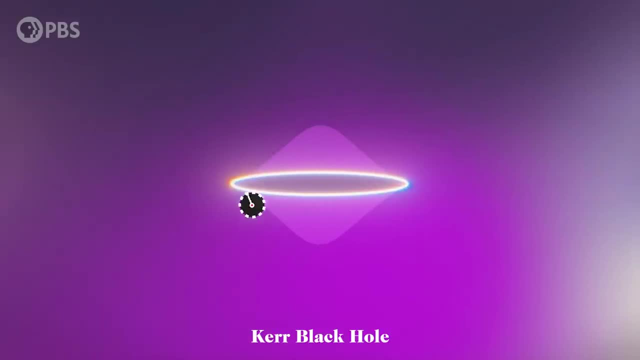 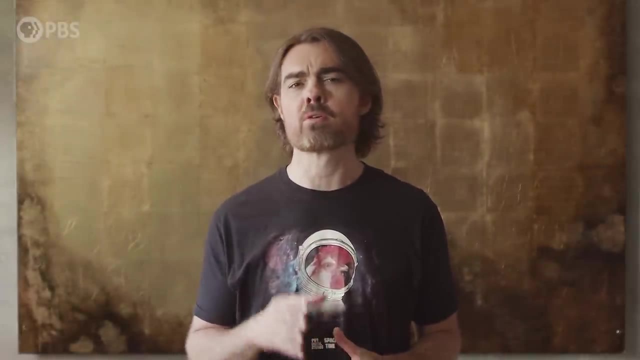 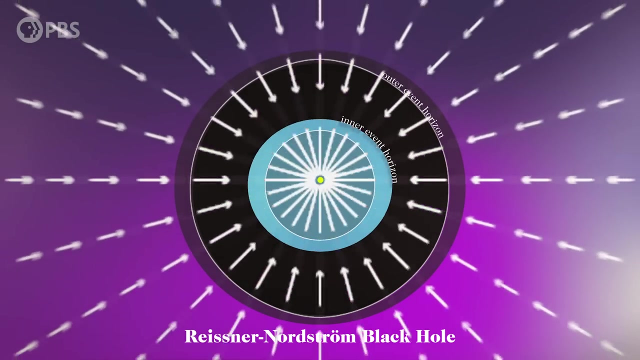 down to the singularity ring, The naked singularity ring. There's a similar situation with the charged black hole which, absent rotation, is described by the Reisner Nordstrom metric: The presence of electric charge at the central singularity which is still point-like in 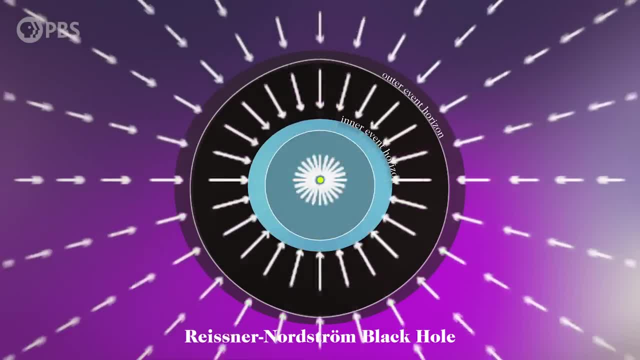 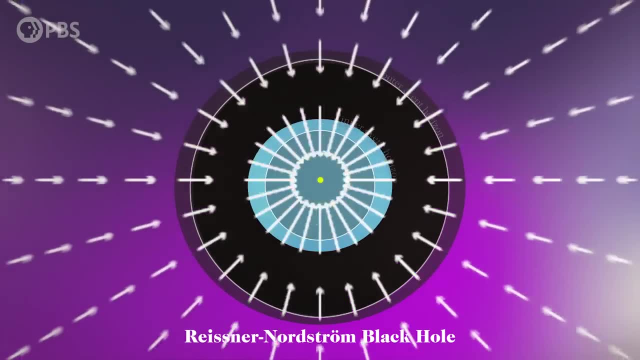 this case results in a rotation of the inner horizon. This results in a negative pressure that again resists the inward pull of gravity. Reisner, Nordstrom: black holes also have an inner horizon interior to which space and time seem normal-ish. 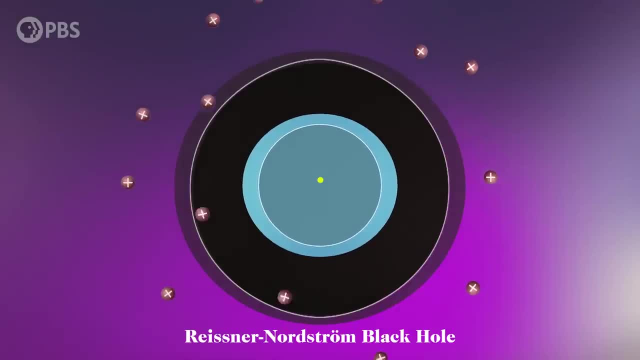 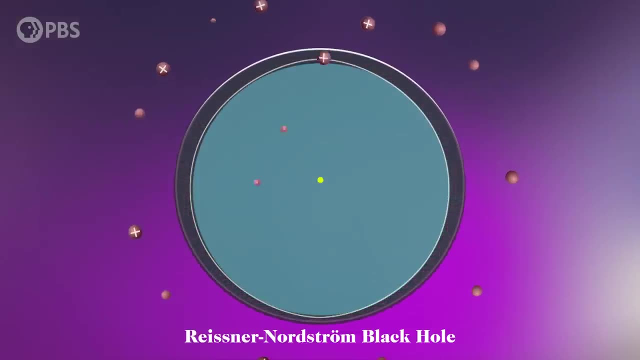 The more electric charge you drop into a black hole, the larger its inner horizon becomes. And, just as with the rotating black hole, at some point the inner and outer horizons become one and vanish, and you're left with a naked singularity. 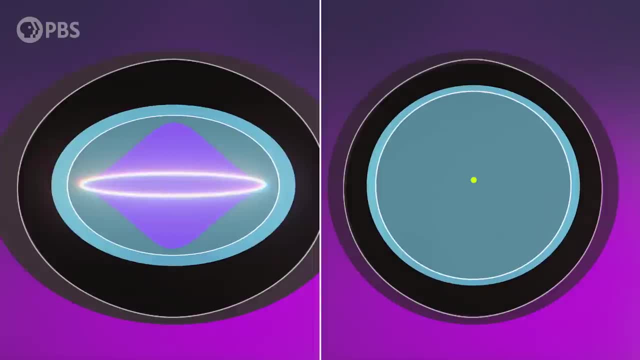 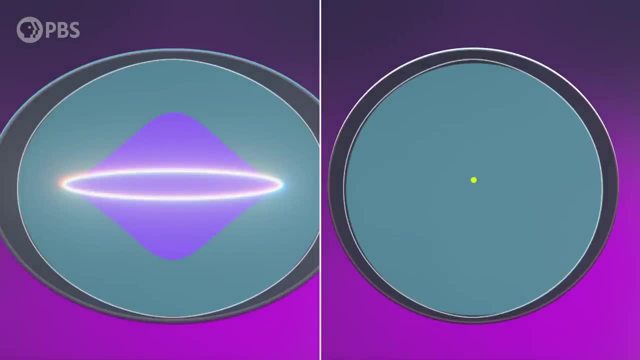 At the tipping point When the inner and outer horizons aren't the same. At the tipping point When the inner and outer horizons are right next to each other, you have what we call an extremal black hole, A black hole with the maximum amount of spin or charge while still having an event horizon. In both cases, the amount of angular momentum or charge that you can fit into the black hole before it becomes extremal depends on its mass. More mass means more inward gravity, and so the black hole can hold more spin and charge before going extremal. 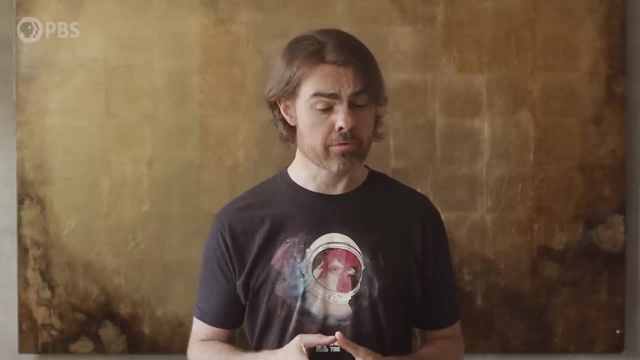 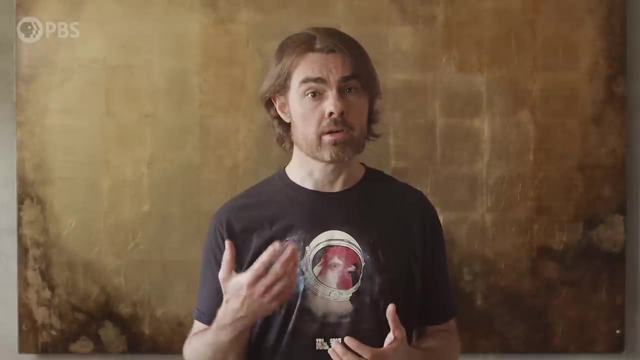 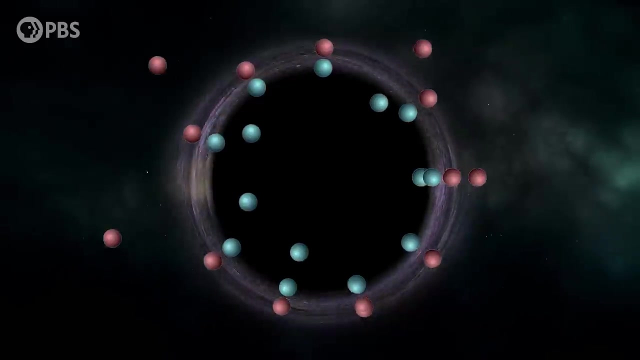 So that is how you make an extreme black hole, Or even perhaps a naked singularity: Just add enough spin or charge to an existing black hole. And actually there is another way to do this in the case of charged black holes. Normal black holes leak away their mass by emitting Hawking radiation. 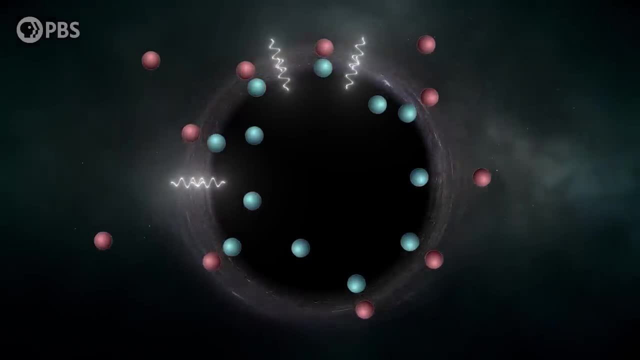 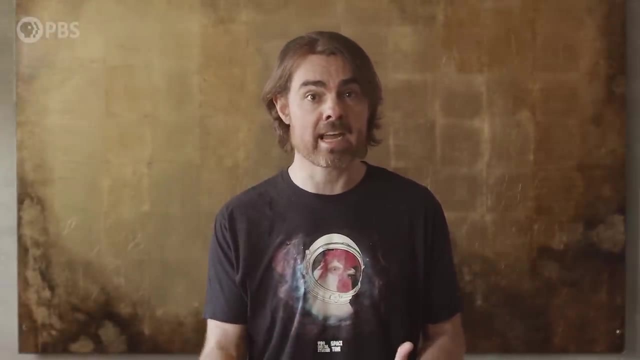 That radiation can be any type of elementary particle, But in the case of the most massive black holes it's mostly just photons. That's because the more massive the black hole, the lower the temperature of the radiation. The Hawking radiation has trouble mustering the energy to make anything but weak photons. 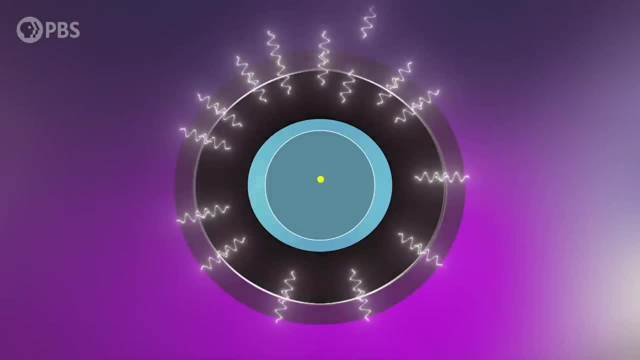 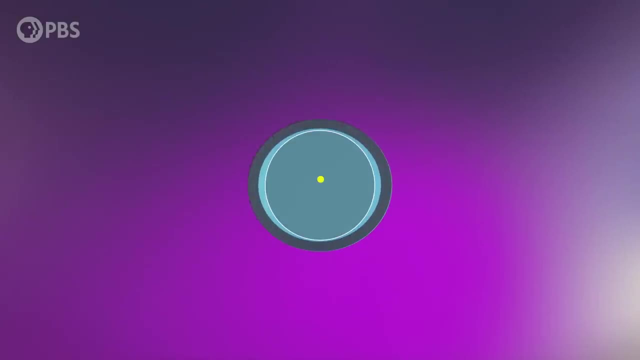 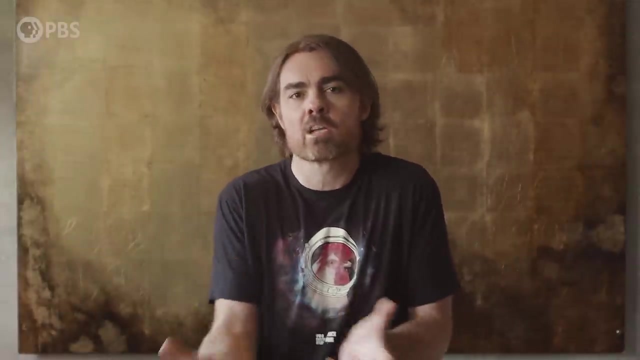 So that means a massive charged black hole will slowly leak away its mass while retaining its charge. The outer event horizon will shrink until it meets the inner horizon and again you have an extremal black hole. This can't happen with rotating black holes, because they leak away their angular momentum. 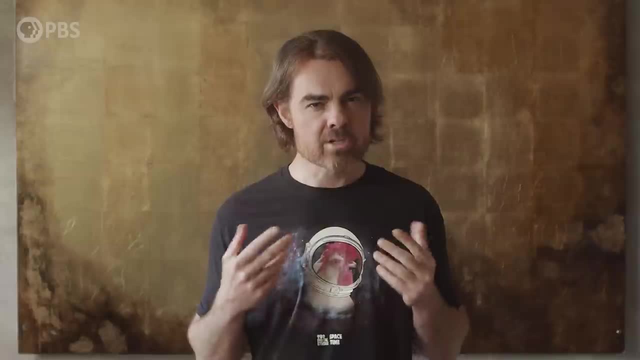 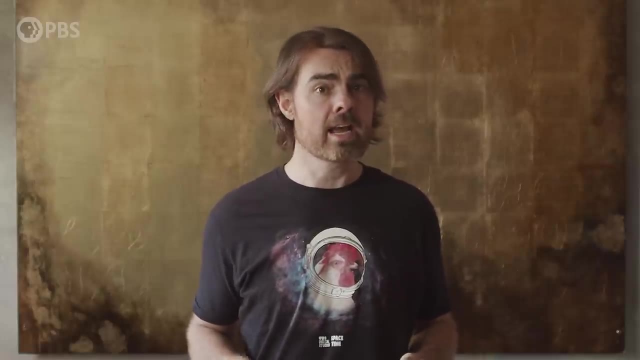 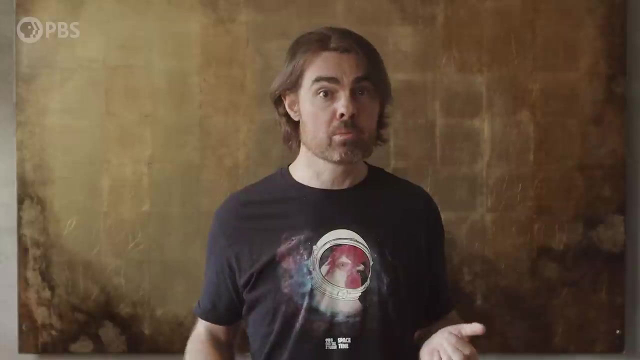 as well as their mass. It's a method that lasts for a very, very long time, if not forever. Hawking radiation is a direct result of there being an event horizon, So naked singularities don't Hawking radiate, and extremal black holes radiate only very. 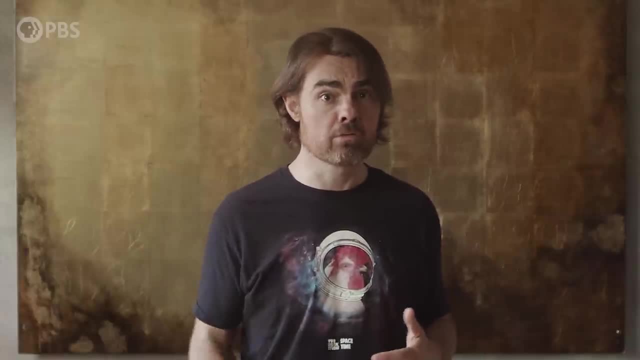 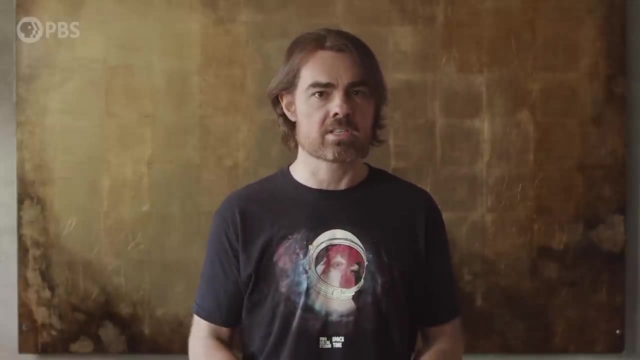 slowly. That leaves us with a strange situation In the far distant future. even if all particles in the universe decay, we may be left with only radiation and these naked charged singularities. So there we have a few recipes for theoretical disaster. Thanks for watching. 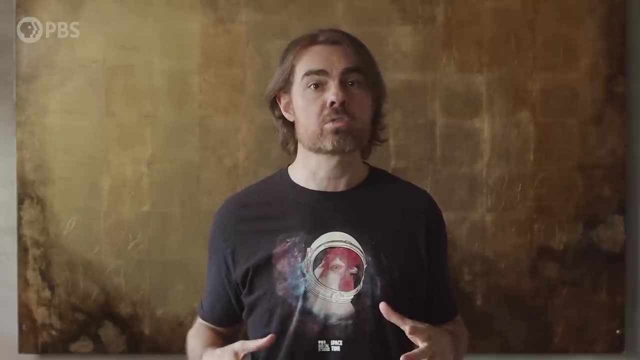 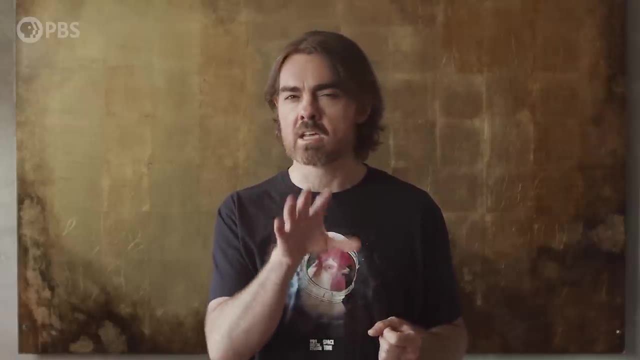 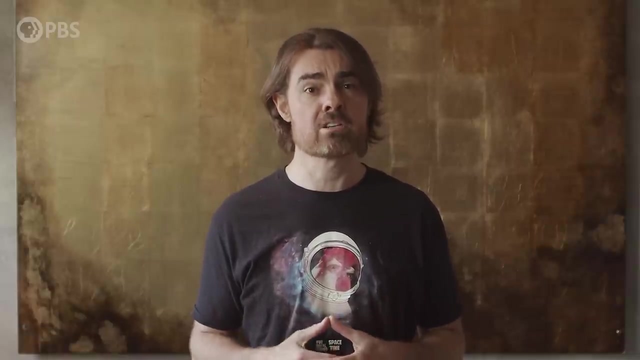 At first glance, it appears that extremal black holes are certainly possible, So why shouldn't it be possible to add a little more spin or charge to produce true naked singularities? The cosmic censorship hypothesis tells us that something will always stop a gravitational singularity being stripped of its event horizon. 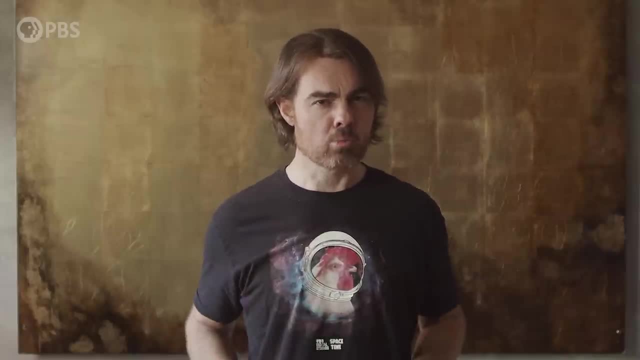 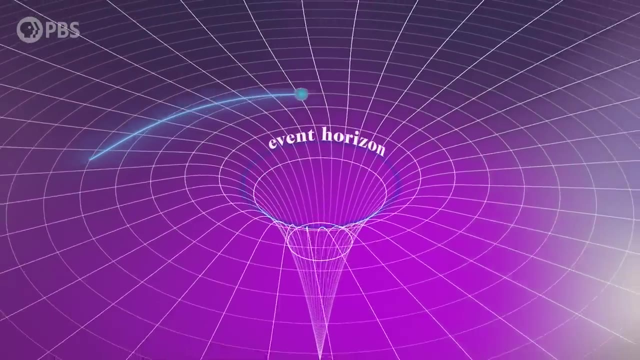 But it doesn't tell us the physical mechanism. Let's look at what we know. Rotating black holes gain their angular momentum from things they swallow. Stuff doesn't normally fall straight away. A black hole spirals in as its orbit decays. 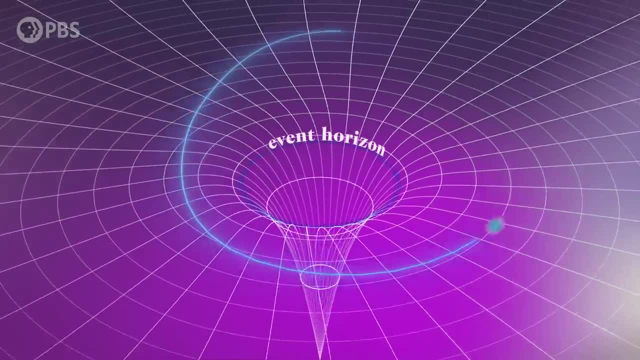 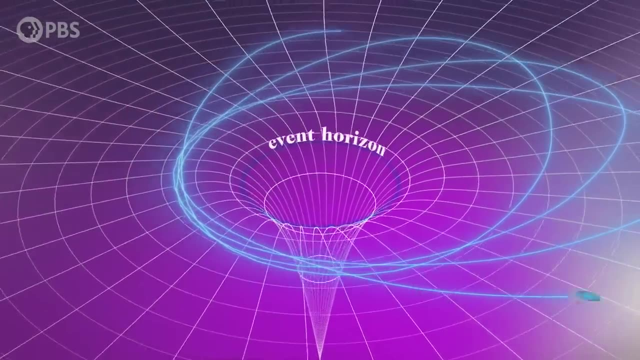 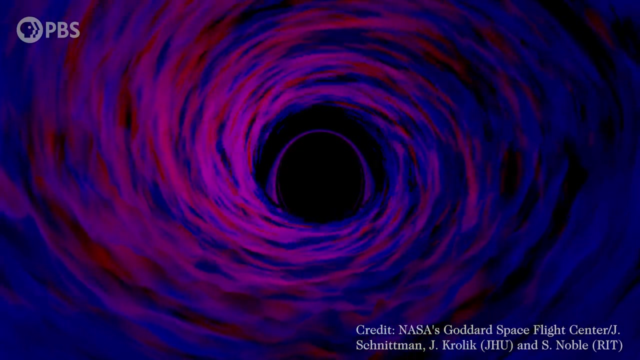 It's that orbital angular momentum that is fed to the black hole. But in order for an object orbiting a black hole to fall into it, it actually has to lose some of that angular momentum, otherwise it would just keep orbiting forever. For example, if there's a disk of gas surrounding the black hole, like in a quasar, then the 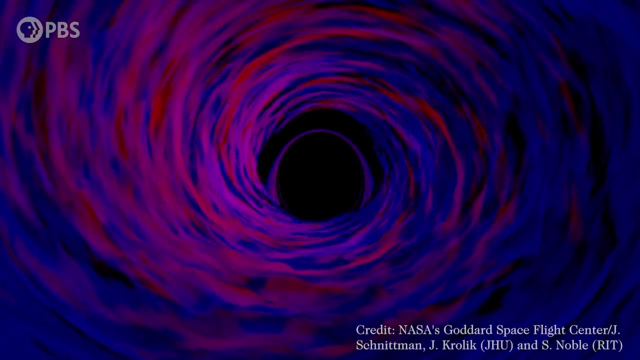 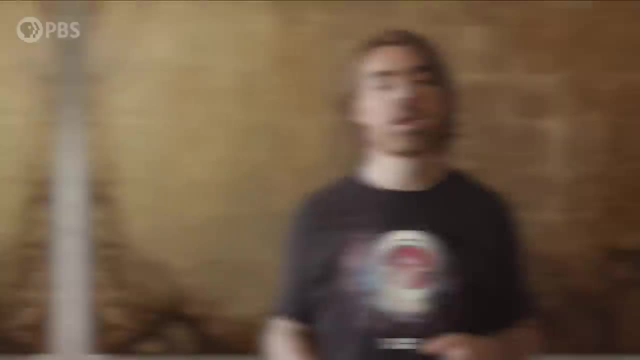 gas only spirals inwards because angular momentum is carried outwards by friction. By the time the gas reaches the black hole, it is lost Much of the angular momentum it started with, And the faster the black hole is rotating, the more angular momentum the gas has to lose. 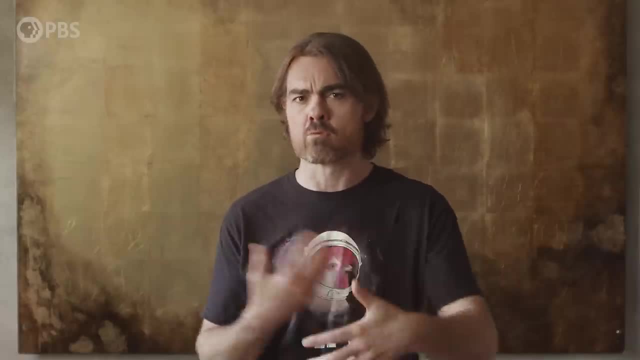 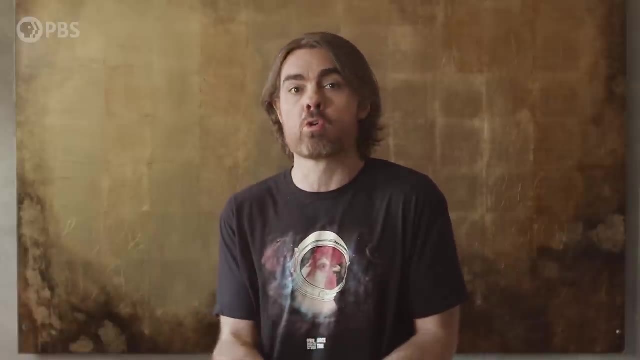 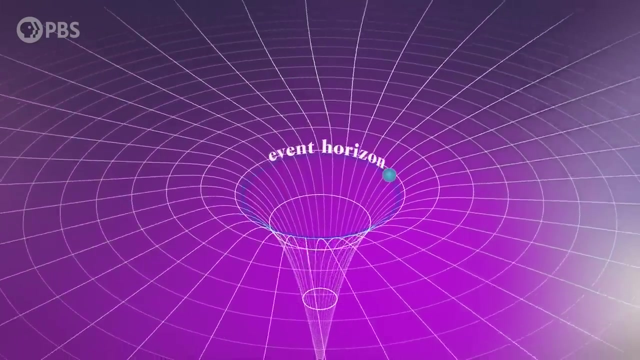 in order to fall in. That's because space gets dragged around a rotating black hole, giving the gas a sort of boost so it can still orbit even with very little of its own angular momentum. In the case of an extremal Kerr black hole, one that's rotating nearly fast enough to 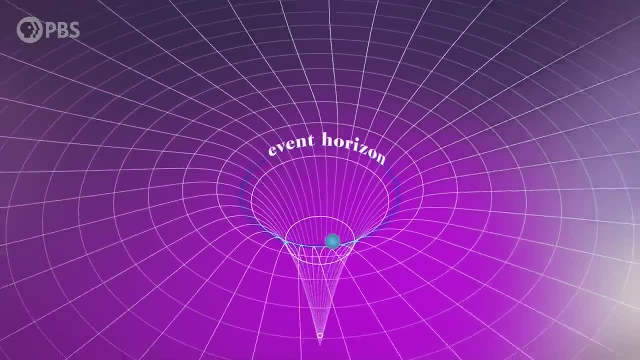 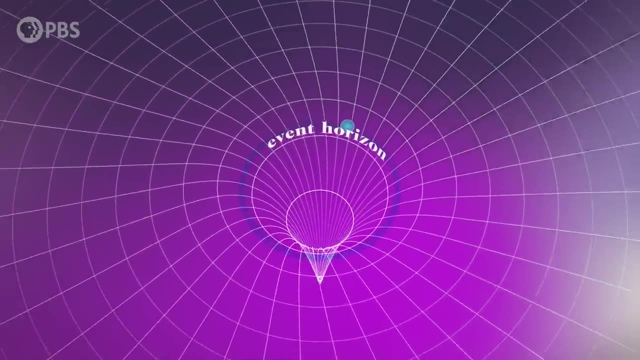 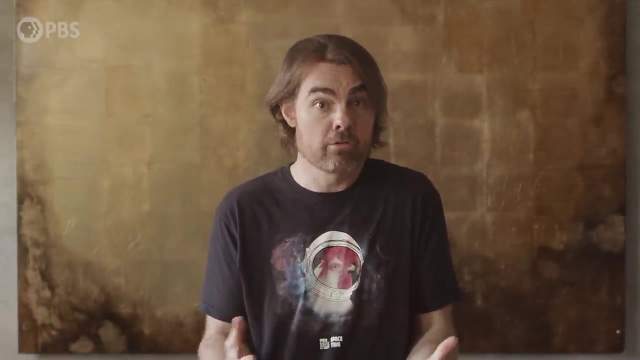 lose its event horizon. the gas near the event horizon orbits entirely. It's entirely riding on the carousel of frame-dragged space and has no angular momentum of its own. Therefore, just on the verge of becoming extremal, the black hole can't gain spin from accretion. 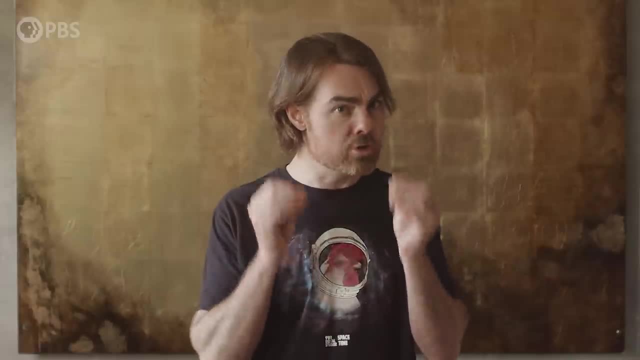 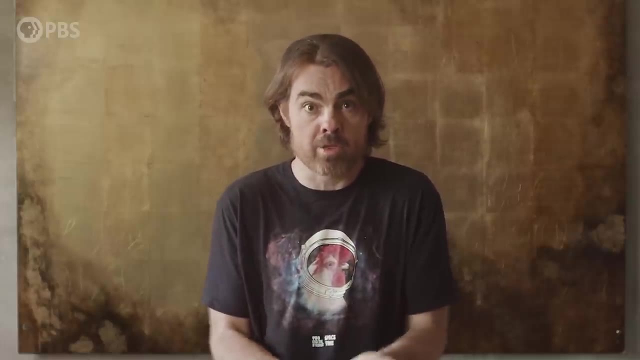 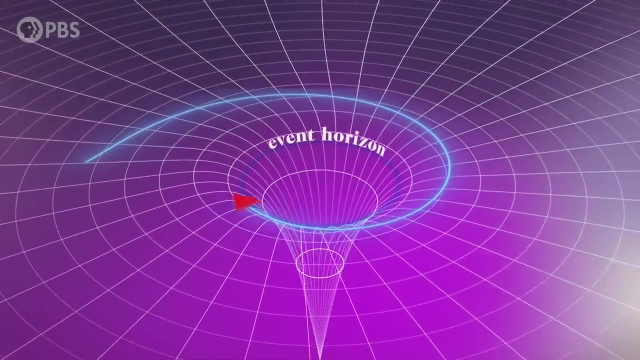 anymore. More generally, there is no trajectory into an extremal rotating black hole that can add angular momentum from the trajectory or the orbit itself. An alternative Is to throw in the gas, Throw in something that's actually spinning itself, so it has intrinsic angular momentum. It's not yet clear whether we can avoid the naked singularity in this case. At any rate, our observations of gravitational waves from colliding black holes and various other methods for estimating black hole spin have not yet revealed a single black hole with a spin high enough to be super-extremal. 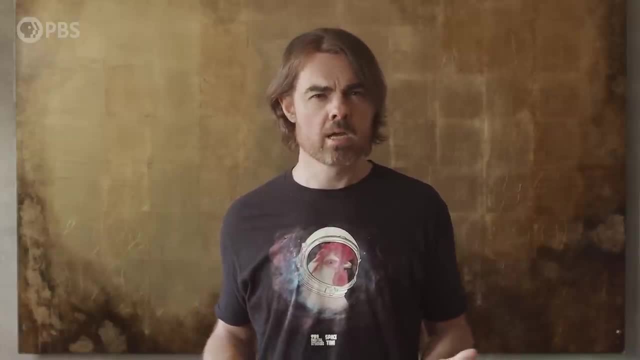 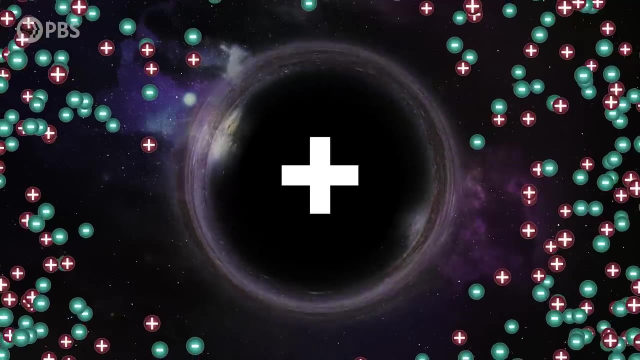 For charged black holes the situation is in some ways easier, But it has its own weirdness. We don't actually expect real astrophysical black holes to retain any significant charge. A charged black hole in the vicinity of any matter would repel light charges and attract. 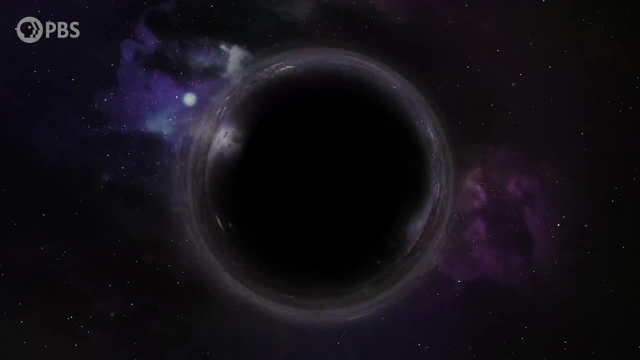 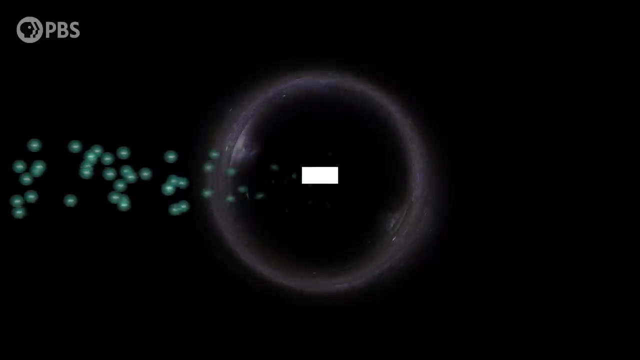 and swallow opposite charges and so quickly neutralize. But imagine we create a charged black hole and isolate it from all other matter. Then surely we can just throw charged particles into the black hole. We have to be careful Because those particles increase the mass of the black hole. 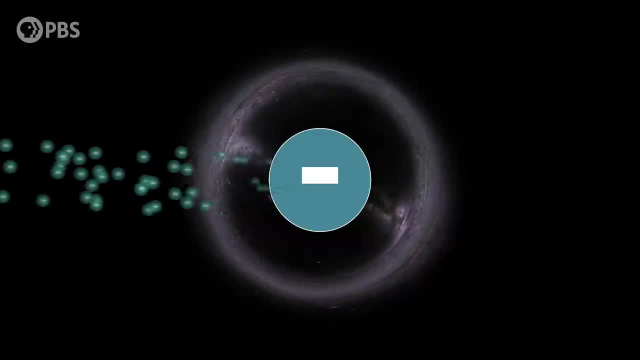 And so we can't just throw charged particles into the black hole. We have to be careful, Because those particles increase the mass of the black hole As well as its charge, And if the mass increases too much it won't go extremal. 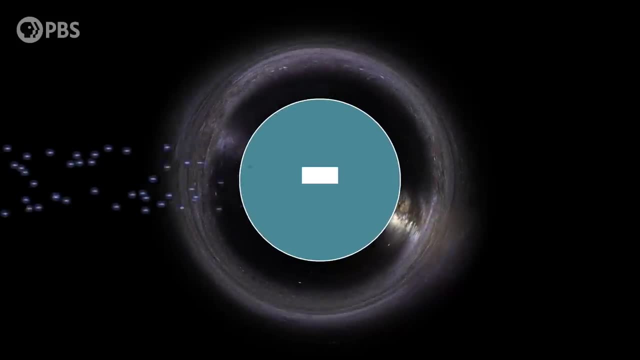 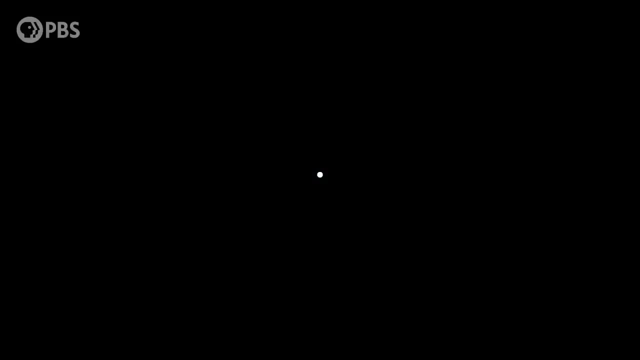 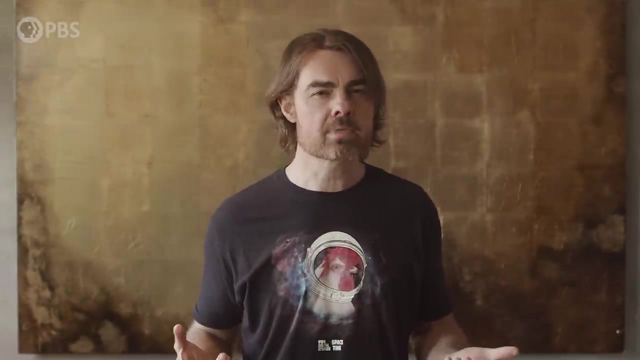 But electrons They have very tiny masses for comparatively large charge. Just factoring the electron's mass, it should be easy to send a black hole over the extremal limit by feeding it a stream of electrons. But here we get to something that seems a bit too neat to be a coincidence. As Einstein taught us, mass and energy are opposed. There's an enormous amount of energy in the electric field of all of those electrons that you smoosh together into the black hole. In fact, the field itself will always generate enough mass to prevent the black hole from. 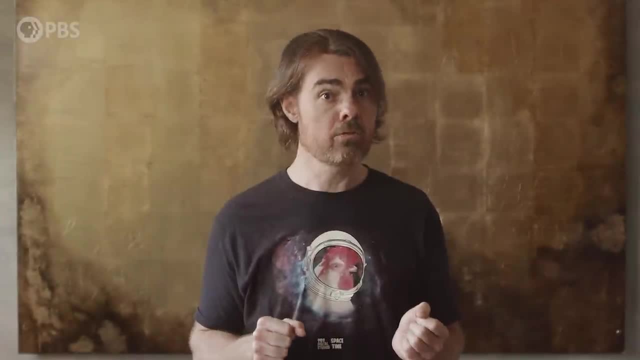 losing its event horizon Once again. the universe appears to have a mechanism to avoid the naked singularity, But there still isn't an underlying understanding of why, or even if the black hole is a black hole, If cosmic censorship must be maintained. 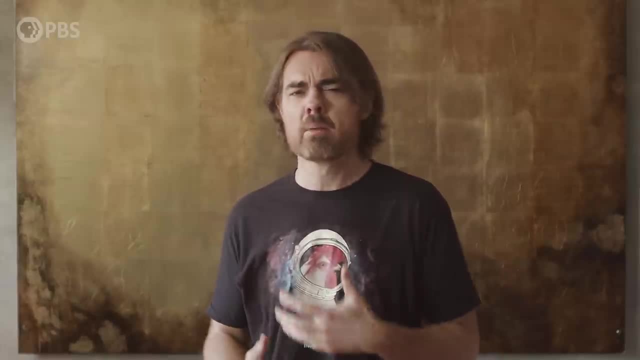 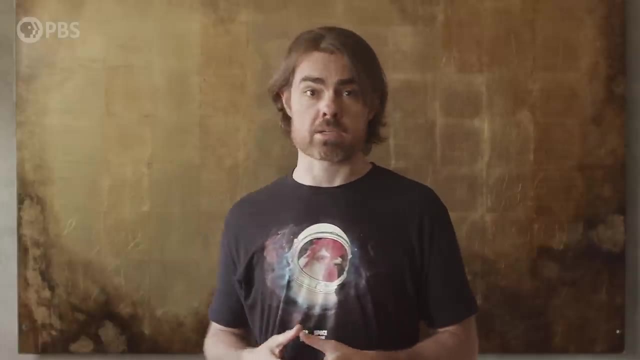 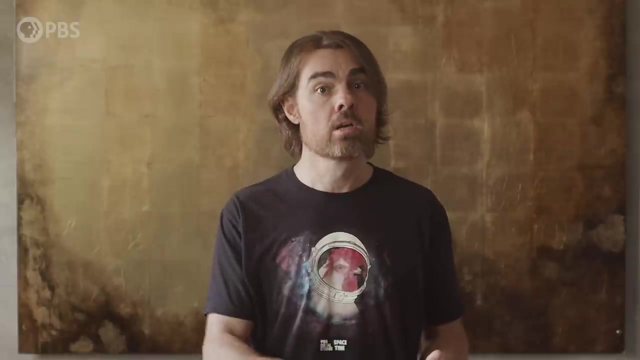 In fact, if you define the cosmic censorship hypothesis in more technical terms, it seems that physics should allow its violation, And that would be a big problem. for physics To really understand that problem and the implications of the cosmic censorship hypothesis being true or not, you'll have to wait for an upcoming deeper dive to witness the horrors. 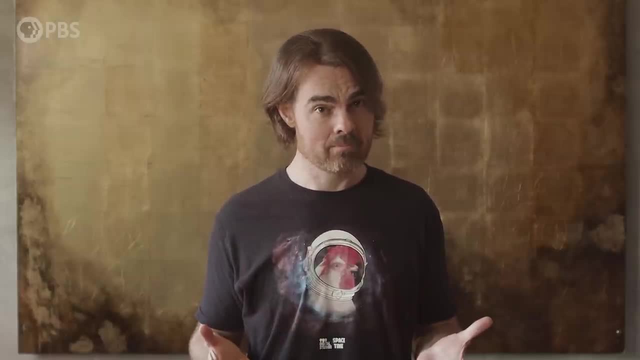 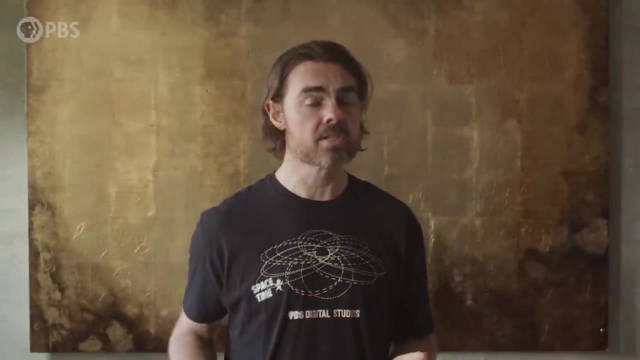 of the cosmically uncensored space, Space time. We missed comment responses last week, so today we're covering two episodes: Building Black Holes in the Lab with Analog Event Horizons and Roger Penrose's Conformal Cyclic Cosmology. 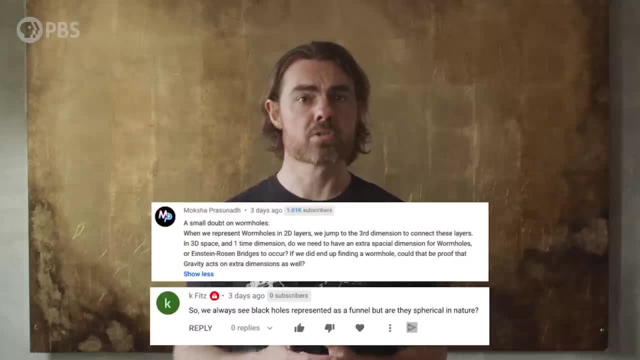 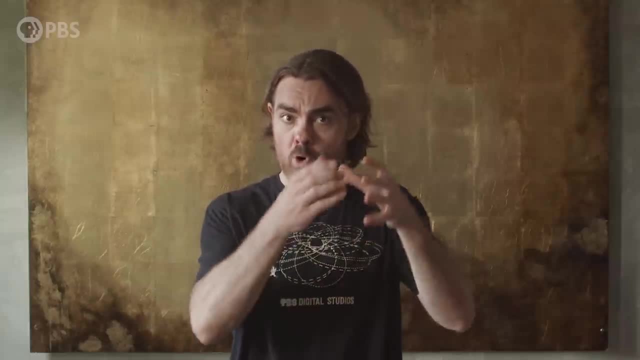 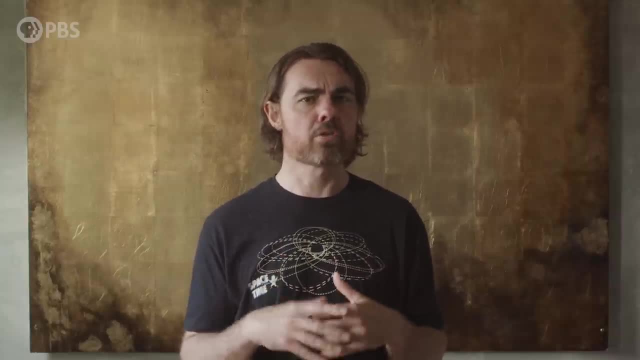 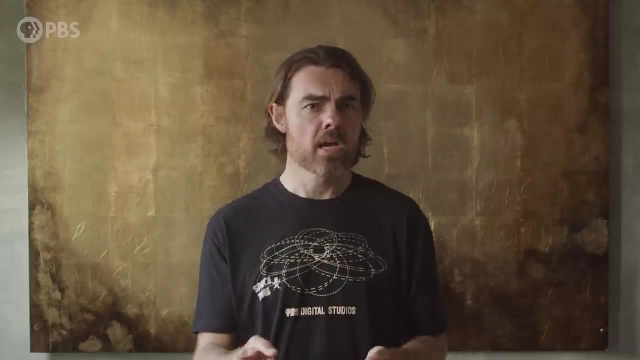 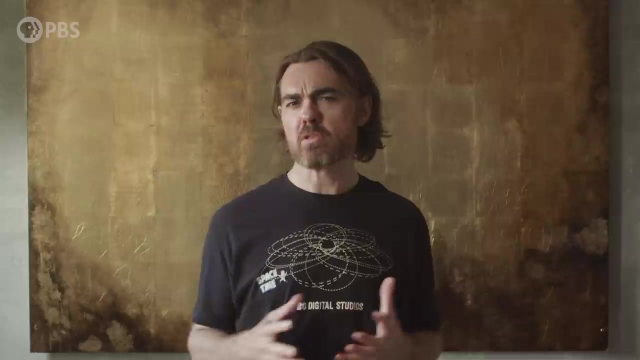 Well, actually in those representations we take 3 dimensional space and take a 2 dimensional slice out of it, so the black hole or wormhole ends are circular instead of spherical. Then the third dimension is just a way to represent the strength of the spatial curvature. 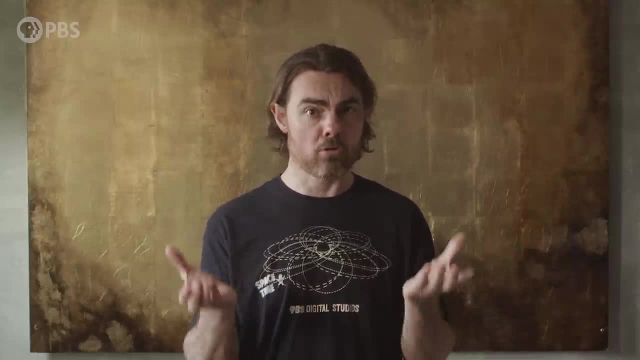 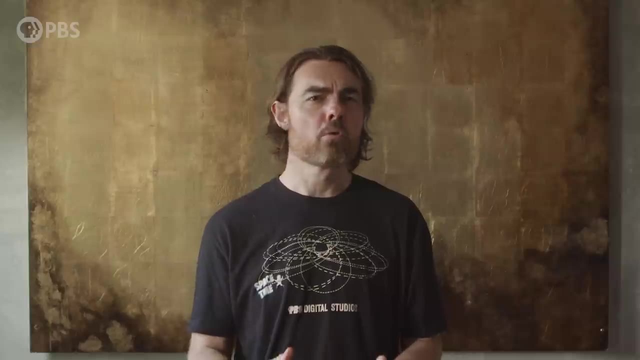 and the connections between different regions. In the case of the black hole funnel, moving towards the bottom means moving towards the central singularity, And the narrowing of the funnel represents extremely curved spacetime, Each ring that you pass as you go down the funnel. 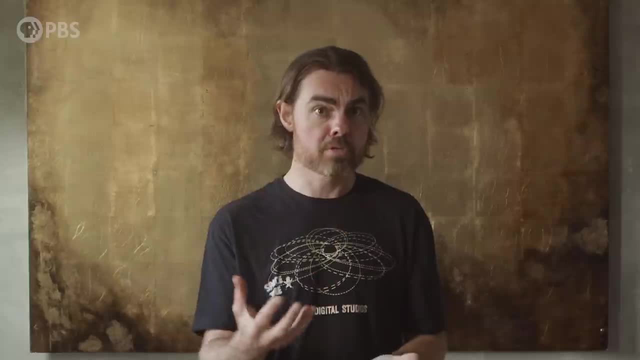 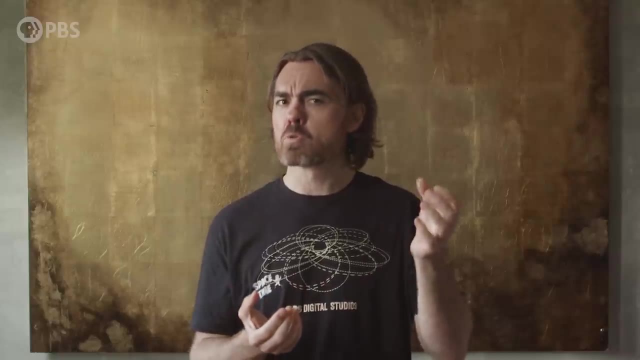 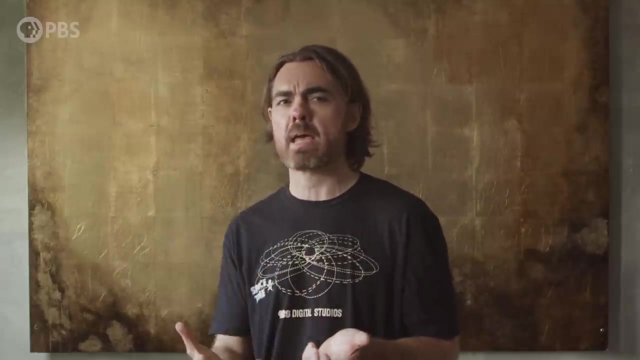 represents crossing a 3D spherical shell. As you approach the singularity, you end up being wrapped entirely around that shell. In the case of the tube between wormhole ends, traveling along the wall of the tube would feel like traveling through a 3D space. 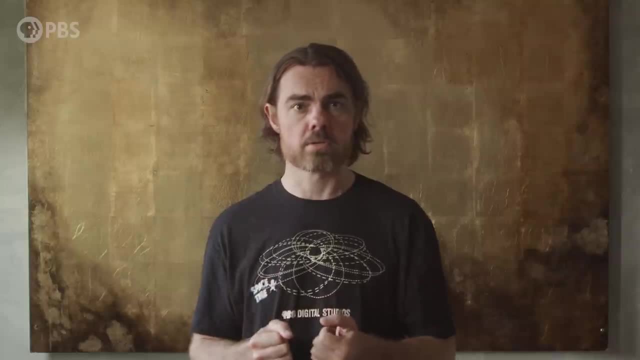 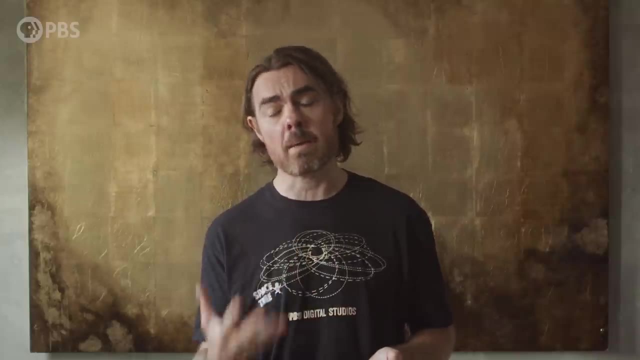 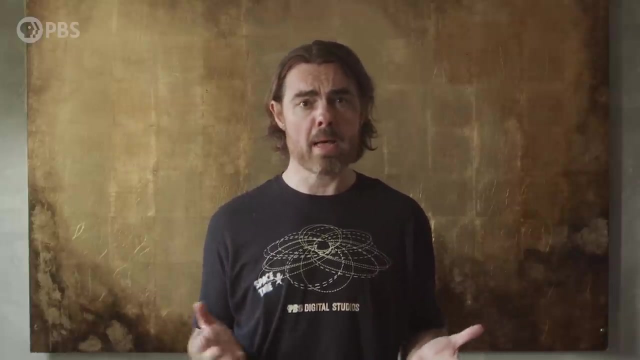 But if you travel around the tube, you get back to where you started. These representations are called embedding diagrams and we went through them in detail in our recent episode on wormholes. OK, on to conformal cyclic cosmology, in which the Big Bang is hypothesized. 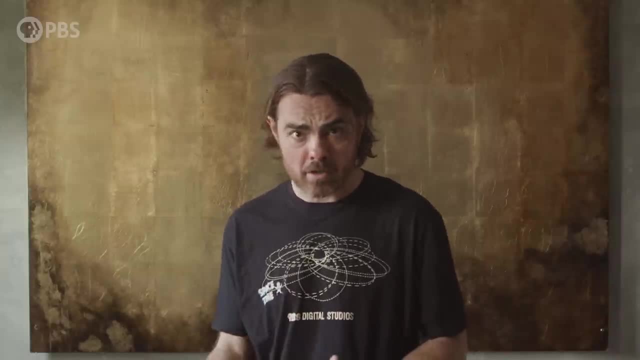 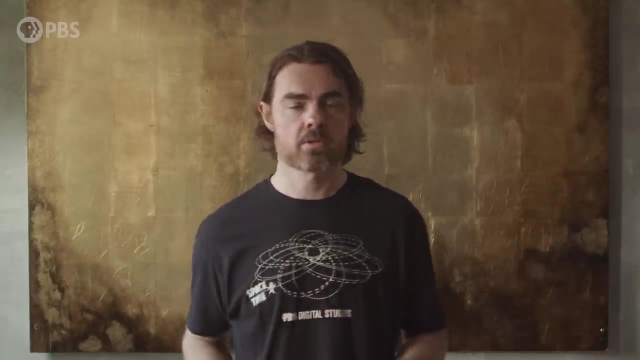 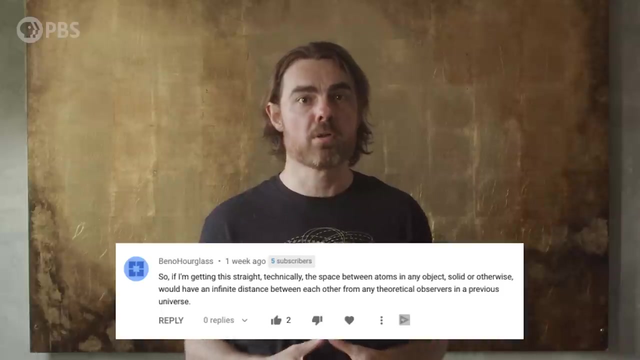 to be the rescaled, infinite late time forever, of a previous universe leading to a potentially endless chain of universes or aeons. Benno Hourglass asks for confirmation of his interpretation of conformal cyclic cosmology. is the space between the atoms in one aeon infinite from the point? 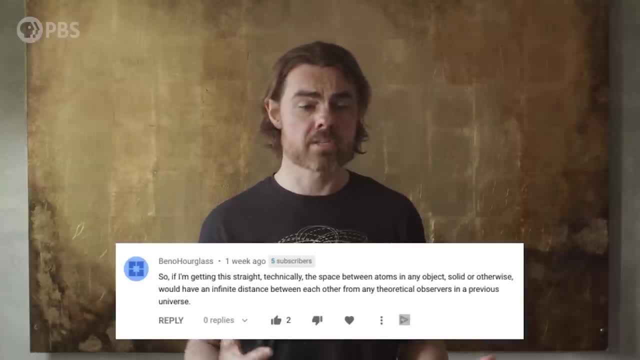 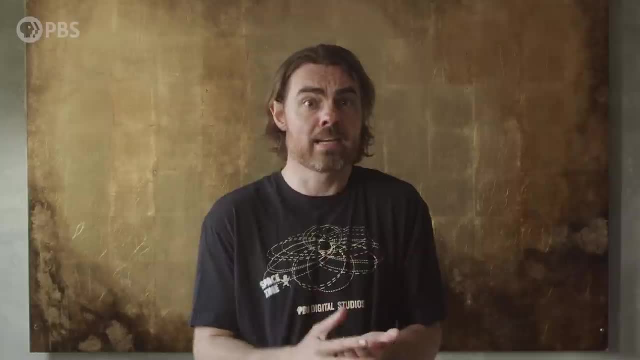 of view of observers from the previous aeon. Well, the answer is essentially yes. Each new, infinitesimally small Big Bang corresponds not just to the very, very large late time of the previous universe, but actually to the conformal infinity of the previous. 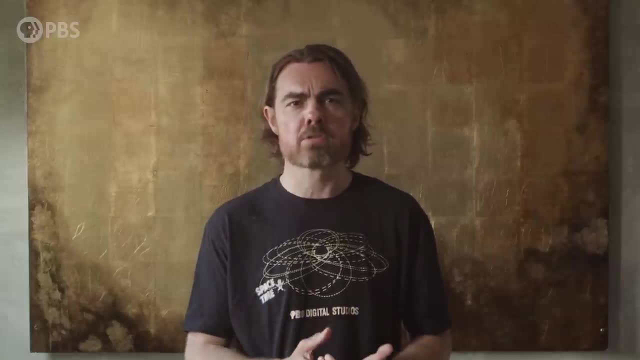 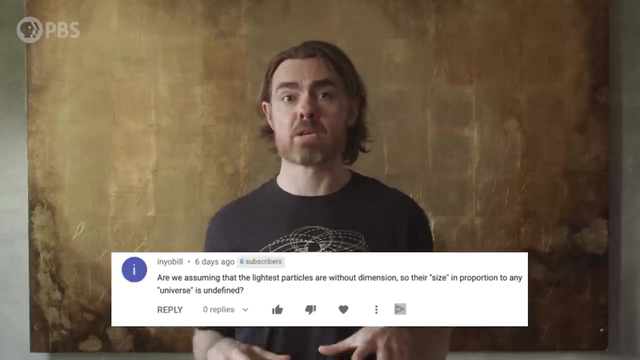 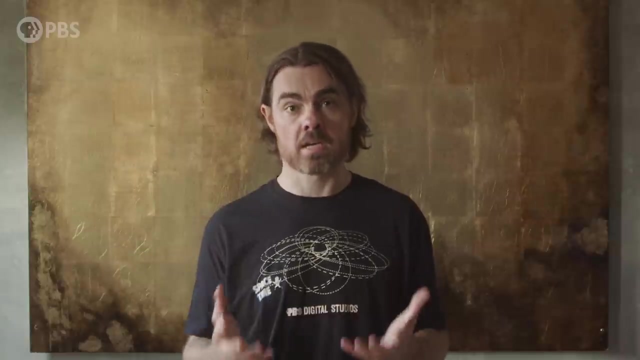 So all the future, The future infinite time of the previous universe added together. Inio Bill asks if we're assuming that the lightest particles are without dimension, so that they have undefined size relative to the universe. Well, I think that's the idea. yes.